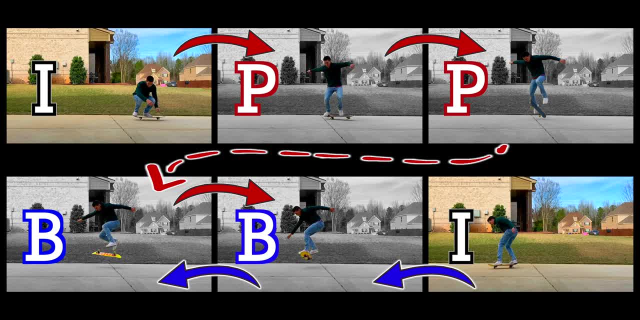 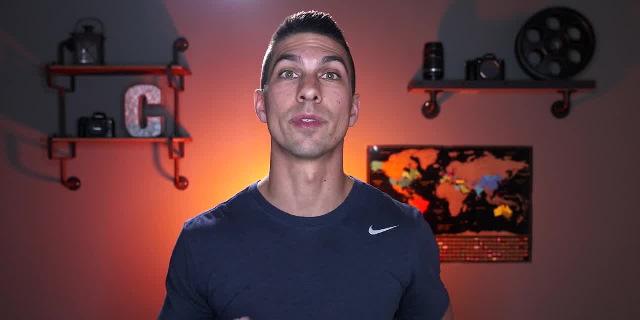 frame information, so that it's basically a blend of the next frame and the previous frame. Simple, right. Well, to put it a little more simply, in a situation like this, where my camera is stationary, the I or the keyframe would record the entire image, whereas the P and the B frames would. 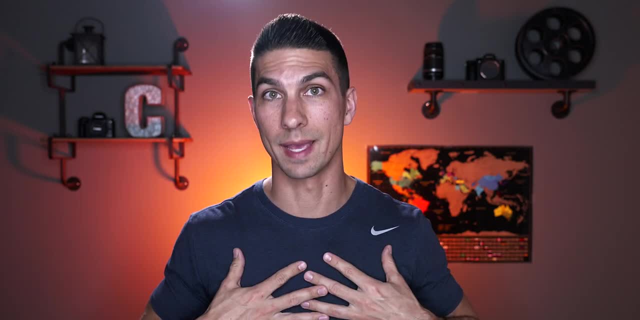 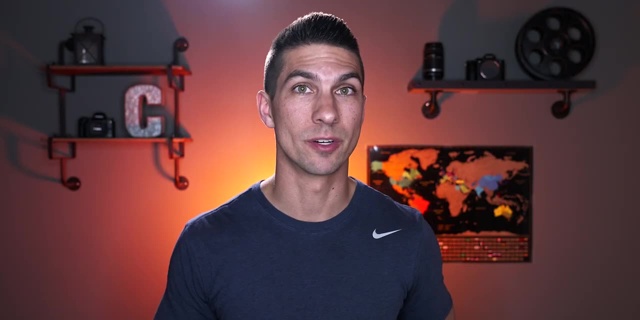 ignore the background and only record the changes in movement that I am making. This results in file sizes up to three times smaller than when recording in the all-I mode, And these all-I and IPB terms are simply Canon's way of expressing these different forms of. 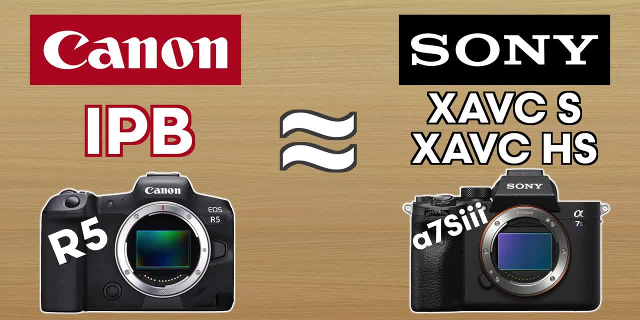 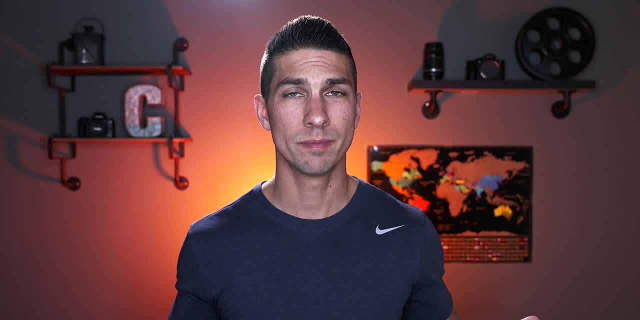 compression, but Sony also has similar options with XAVC-S being like IPB and XAVC-SI being like all-I. Does that make sense so far? Let me know if you're still with me by leaving a thumbs-up. If you liked this video, be sure to give it a thumbs-up and subscribe to my channel for. 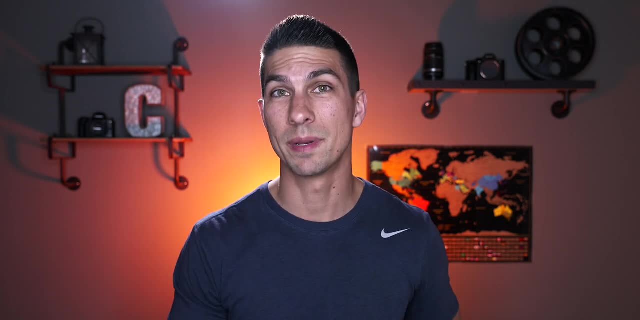 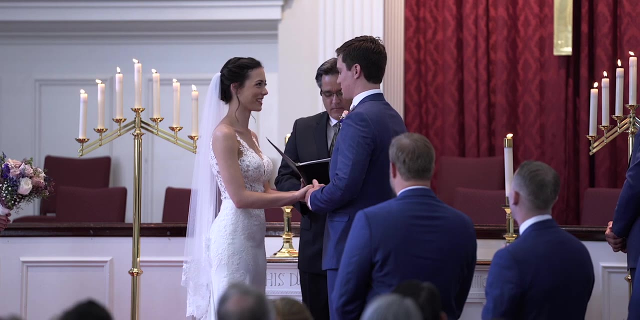 more videos like this. Now that we know what's happening with these different forms of compression, let's look at times when you'd want to use one over the other. IPB is more suited to times when your camera is stationary is when filming something like. 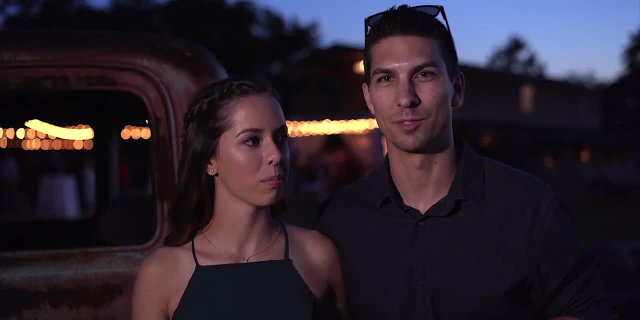 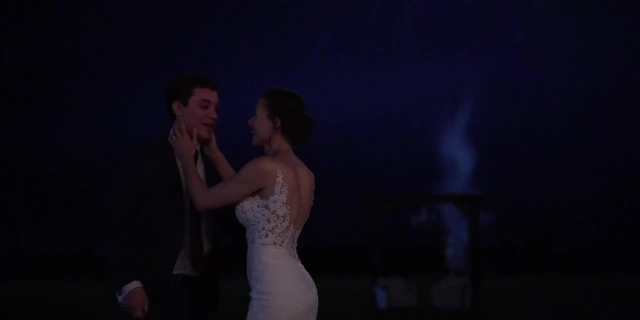 a wedding ceremony or an interview where there isn't a lot of movement going on in the frame. But when you start moving to more dynamic shots with lots of camera movement or lots of subject movement within the frame, or even shooting darker scenes, all-I will guarantee. 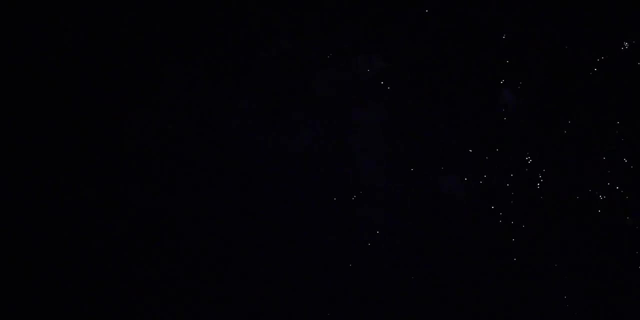 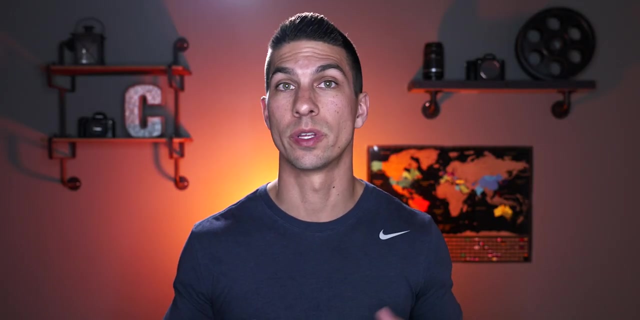 the highest quality, along with the larger file sizes, because every frame is being treated as one of those keyframes rather than using predictions. And another thing to consider when choosing which compression mode you're going to use for shooting is your computer's processing power. And even though the all-I files are about three times as big as the IPB files, the lower 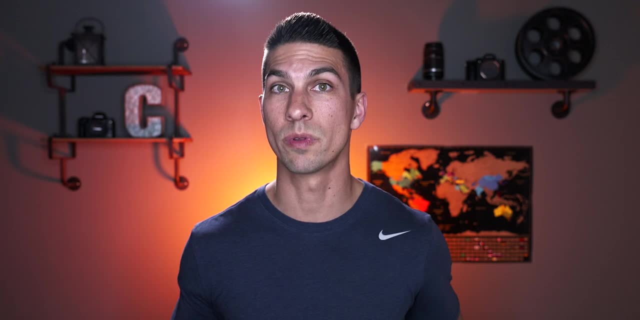 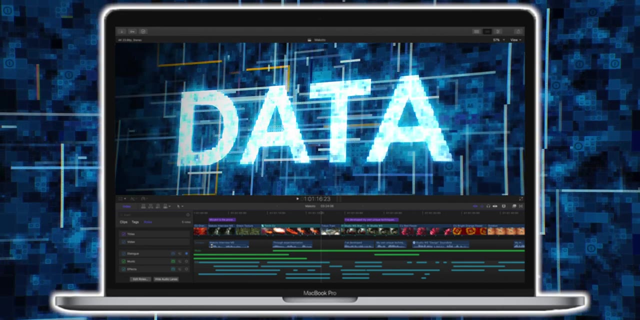 compression of the all-I frames makes editing run much smoother than when using IPB frames. This is because the decompression of the IPB frames involves more complicated calculations in decoding all the predicted and bidirectional frames just to show a single frame. And when using all-I, you won't have to worry about the fact that you're not going to. 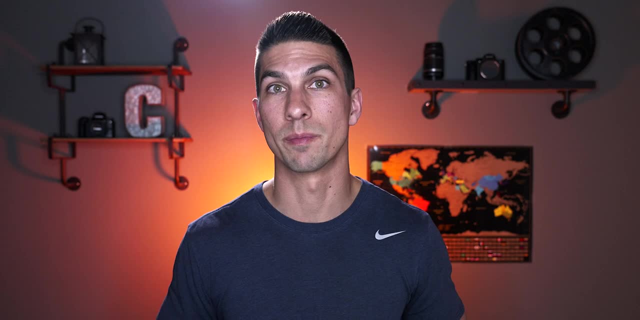 be able to use all of those keyframes. You'll have issues with motion artifacts caused by incorrect inner frame compression. that can happen with IPB files And also if you plan on doing a lot of color grading or working with green screen, then 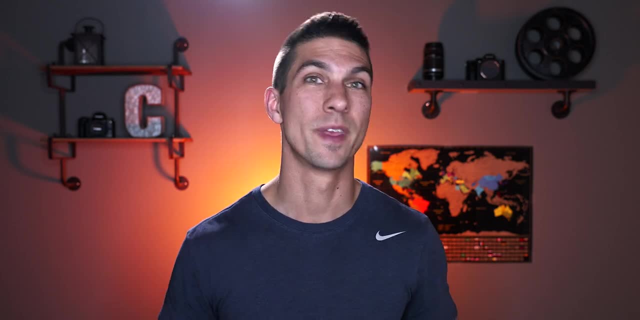 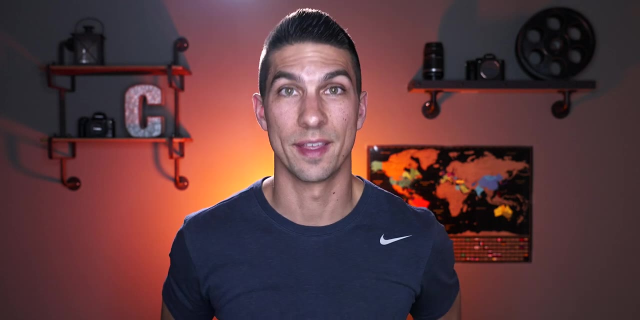 using all-I can make this process much simpler for you, But I hope this made sense and if this video was helpful, then please help me out by leaving a like. subscribe if you haven't, and I'll see you in the next one.